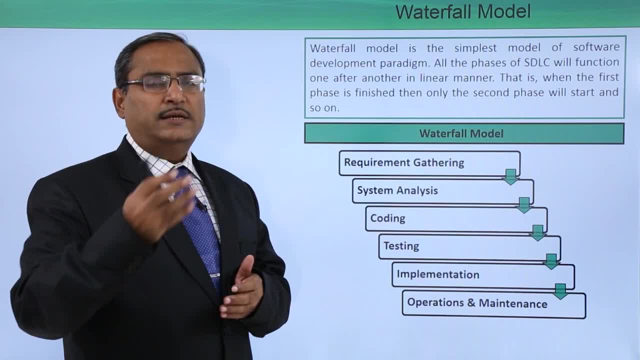 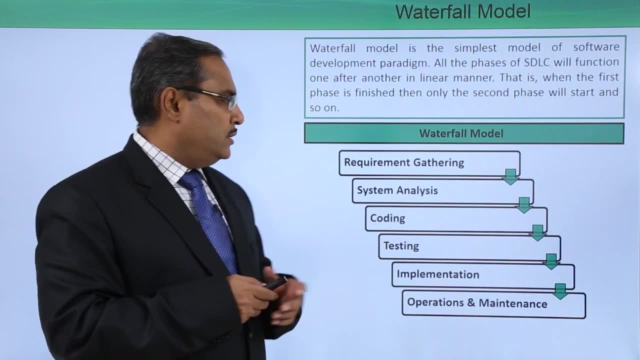 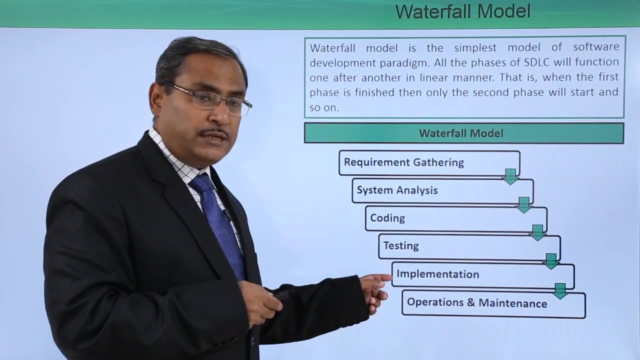 will start, and so on. In this way, the phase wise, the respective software development will be done. So here we have considered some of the steps. So we recommend gathering, system analysis, then going for coding, then testing, then implementation, then operations and maintenance. So in this way we have gone through In. 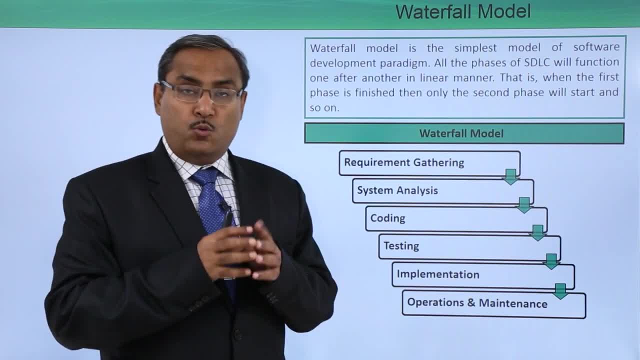 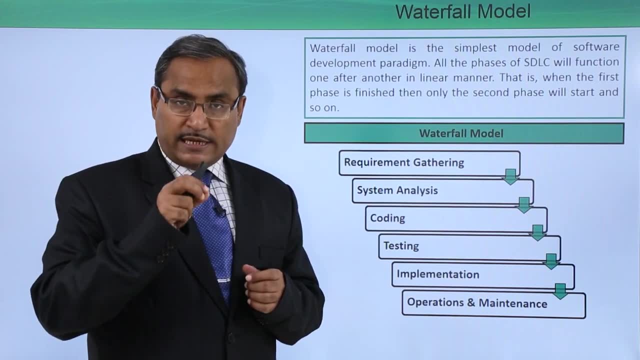 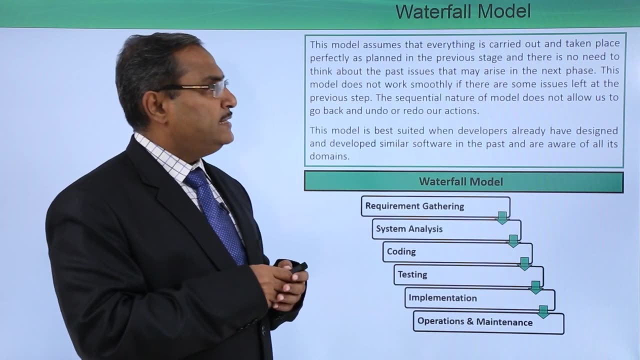 our earlier video in our software development paradigm, we have discussed all these respective phases, what are their purposes and what are the main objective in each and every phase. You can watch that video also, And we have discussed last time as well. So the first phase is that's called call. 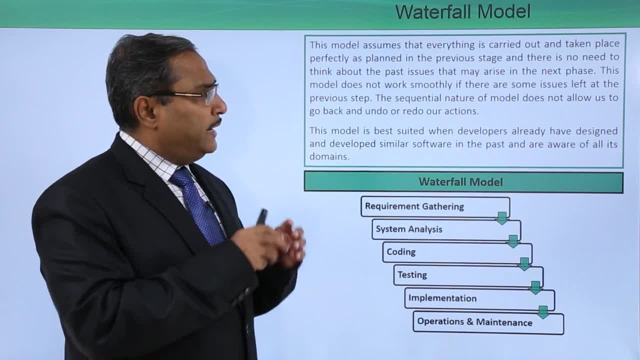 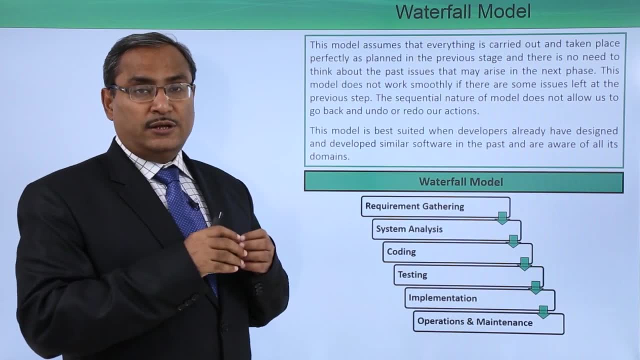 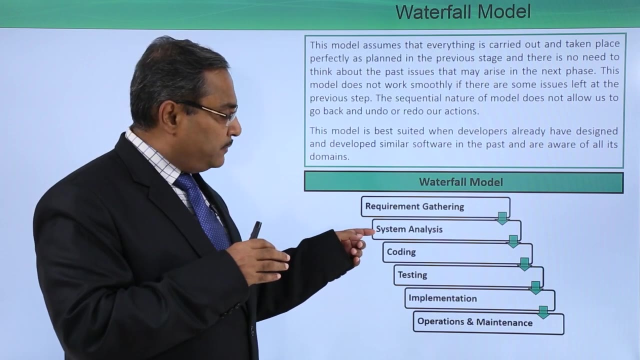 KYP or call Sky way. See, All that will happen is that trigger a forward call And then trigger composed call to the point, and If I go to this point it will not oriented at the cineral bend to this. 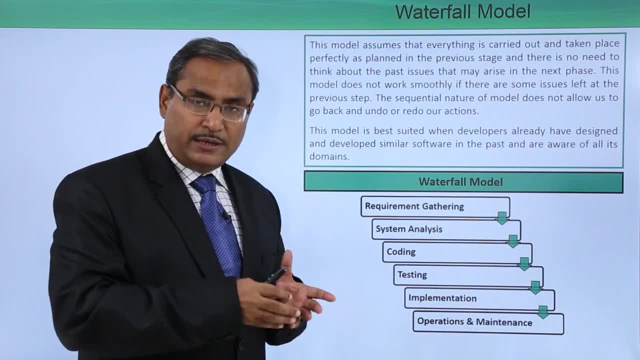 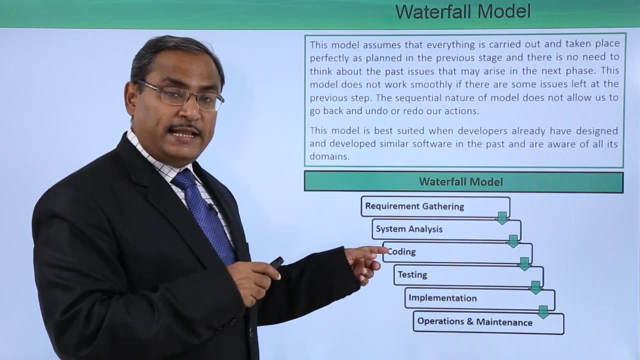 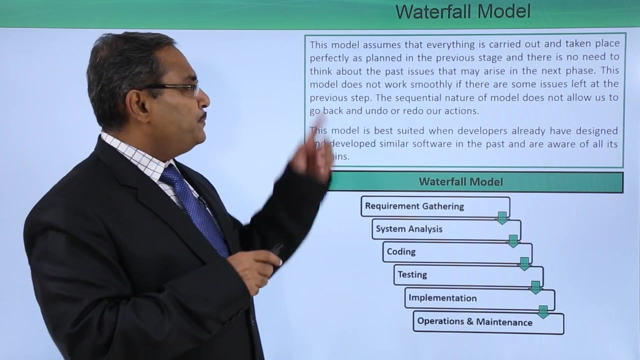 point I should say: what about the issues we will be having here? we should fix it. then you should come to the next phase And in this particular phase we should not consider any issue related with the previous phase or phases. This model does not work smoothly. if there are some issues, 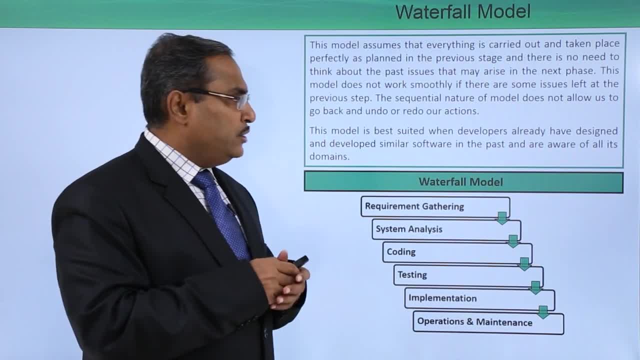 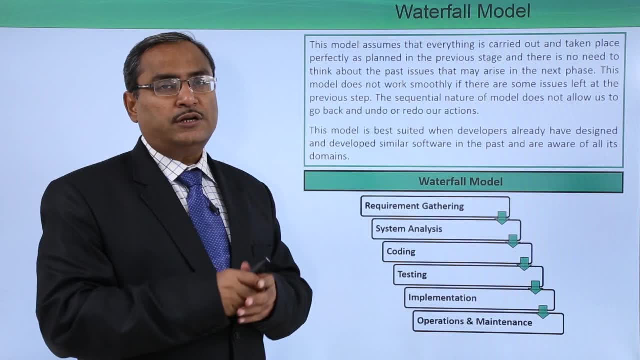 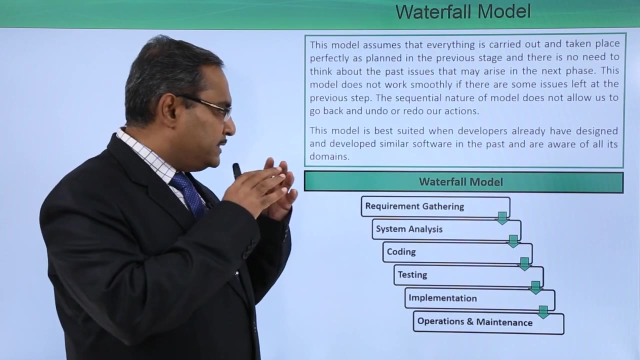 left at the previous step. The sequential nature of model does not allow us to go back and undo or redo our action, So that is the main feature of this waterfall model. This model is best suited when developers already have the designed and developed similar software. 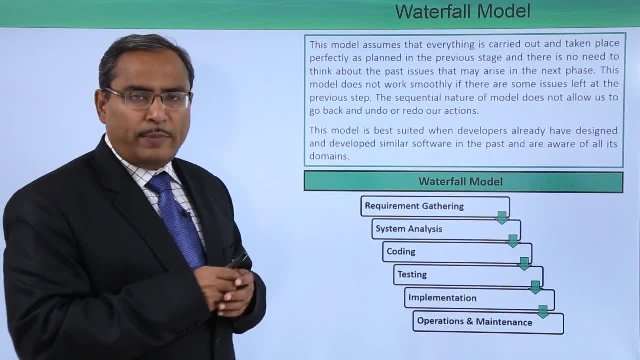 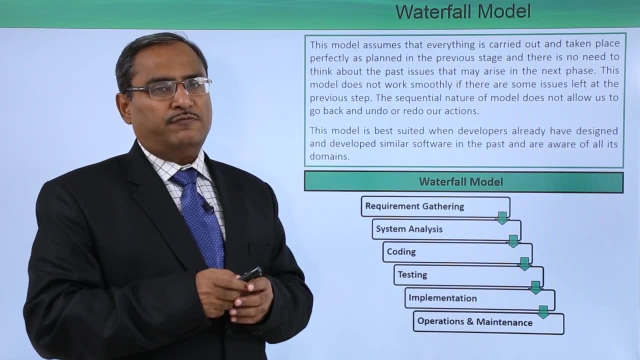 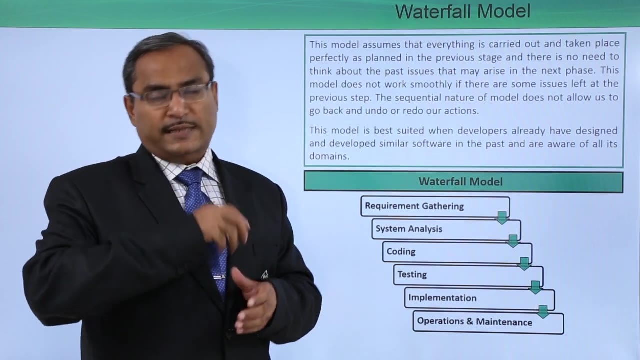 in the past and are aware of all its domains. When the requirements are known at front, beforehand, then only this particular waterfall model can be applied, And if the developers are having the prior experience developing the software in the same domain, then this waterfall model can be utilized. 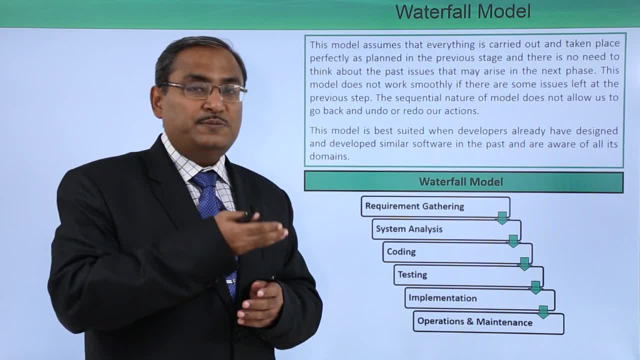 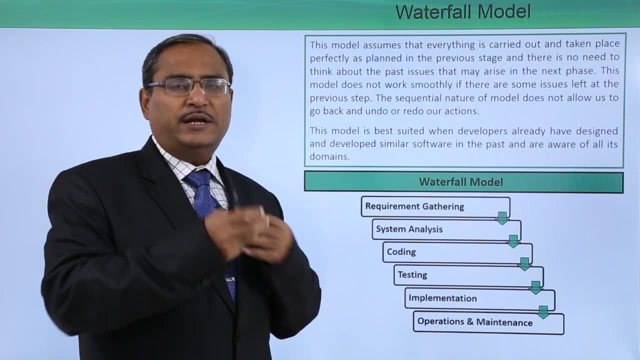 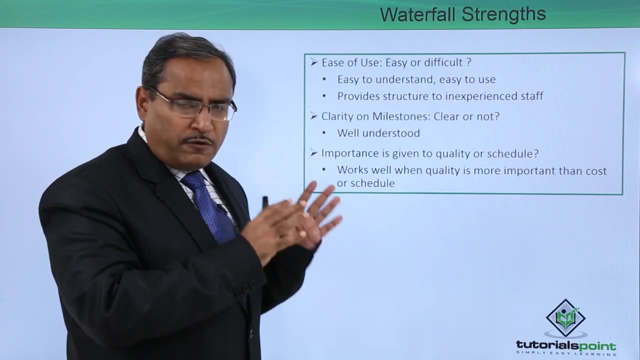 can be implemented. Otherwise, you see, you cannot retrace back, there is. there is no scope to going back to the previous step or phase and do some rework and do and undo there. that is not possible. Now let us discuss waterfall strengths. So in case of waterfall strengths, the first question is that: ease of use, easy or difficult? 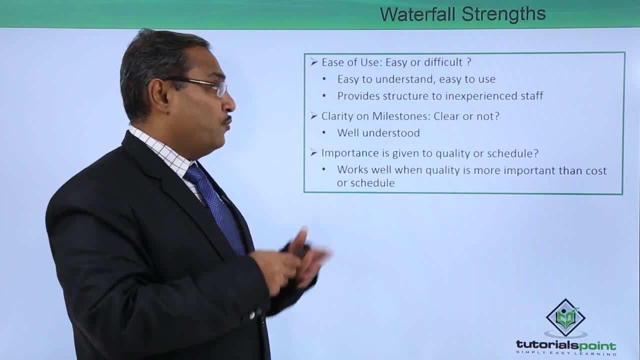 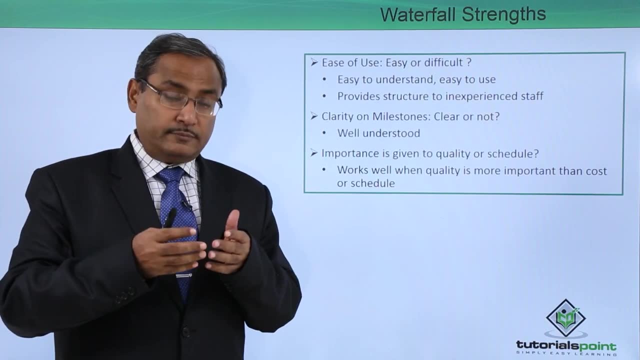 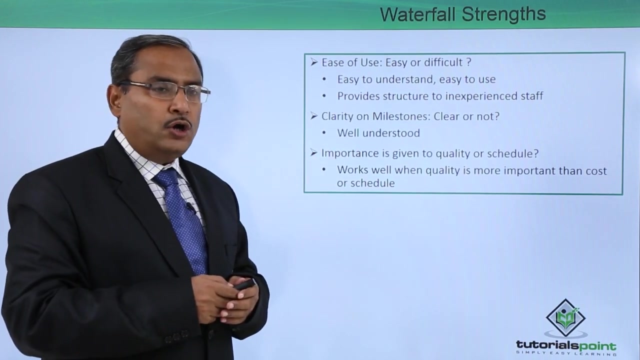 the answer is easy to understand and easy to use and provides structure to inexperienced staff. for for the freshers in the project management in the software development projects, is waterfall model is suitable? clarity or milestones? clear or not? answer is well understood. milestones will segregate between one phase to another phase. 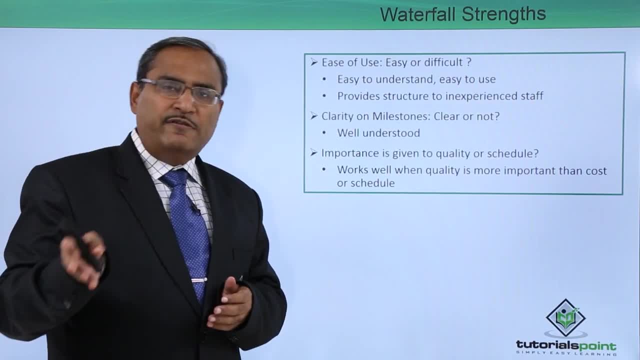 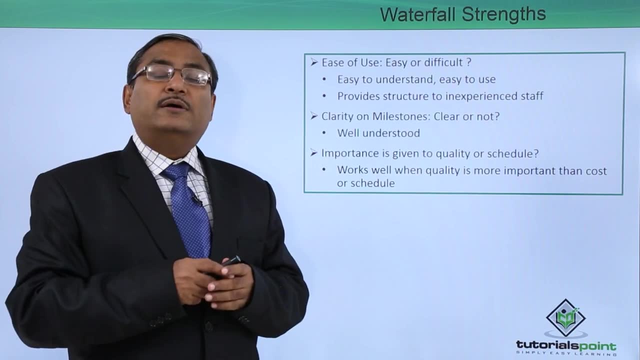 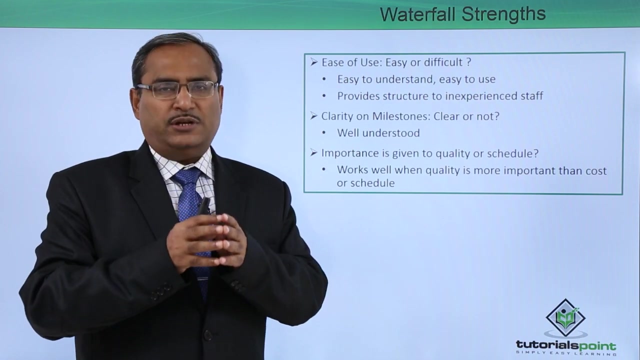 So whenever we are crossing one milestone, that means we cannot revert back, we cannot retrace our path again. So in our project management this milestone will be denoted by activity with the duration 0. but here, actually, this milestone is denoting that differentiation or the segregation between 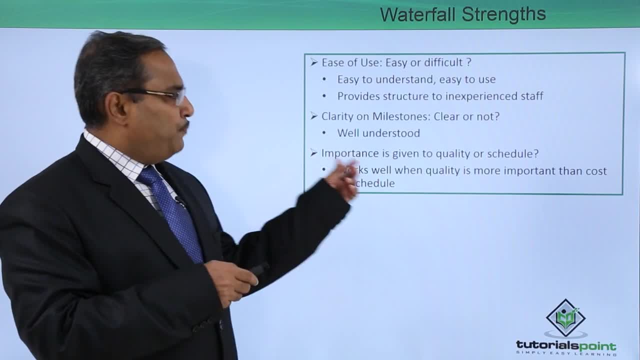 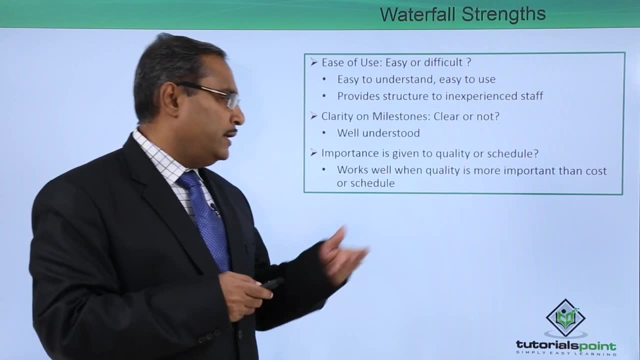 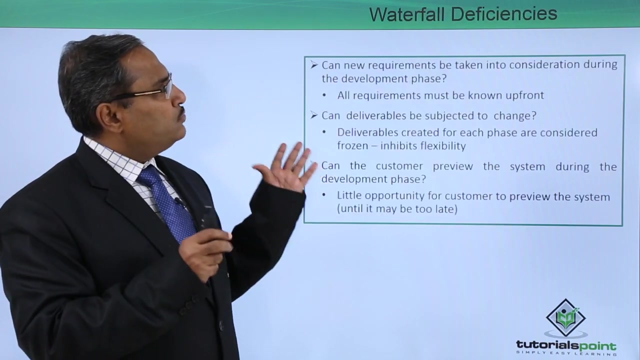 two adjacent consecutive phases. So importance is given to quality or on schedule. the answer is: works well when the quality is more important than cost or schedule. So this is. these are the strengths of waterfall model. So now let us go for the waterfall deficiencies. 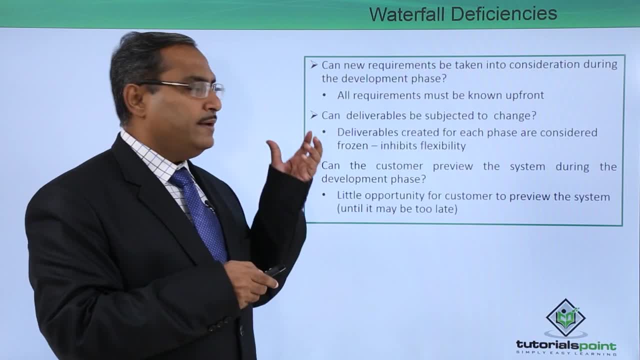 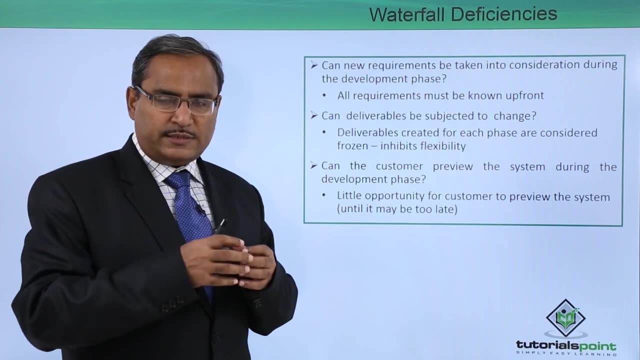 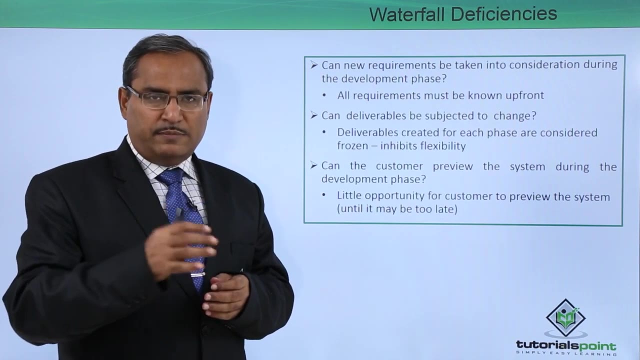 Can new requirements be taken into consideration during the development phase? So when the when the software is getting developed, can it incorporate the new change requests new requirements? Answer is: all requirements must be known upfront beforehand. So when the system is getting developed, when the software system is getting developed, no. 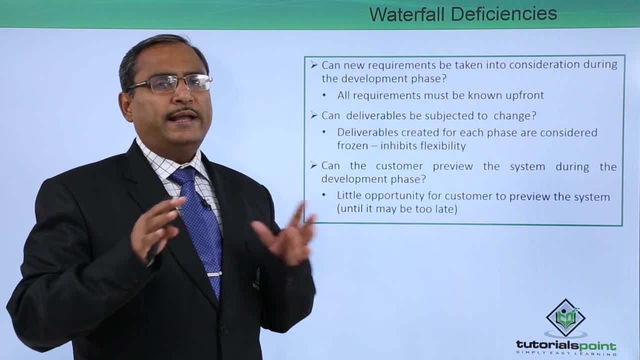 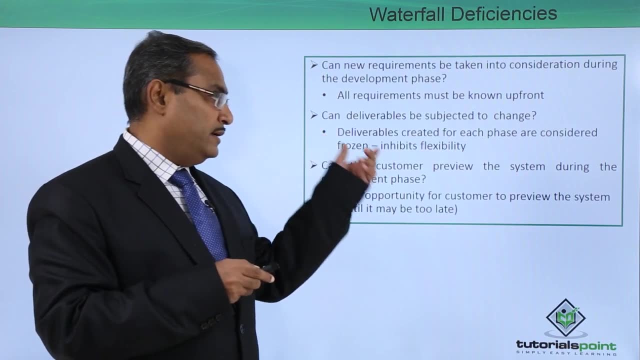 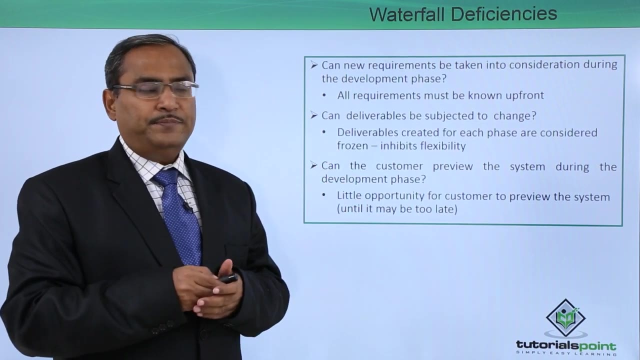 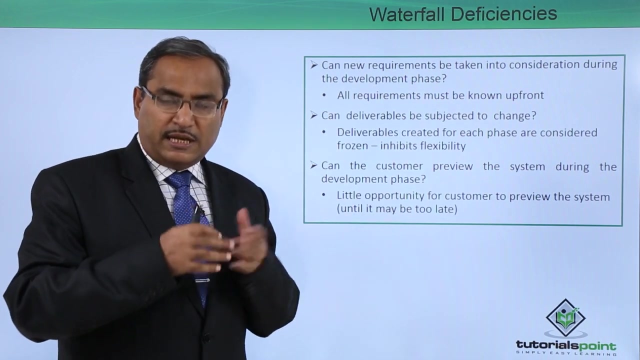 new change requests or no new requirements can be entertained. Can deliverables be subjected to change? answer is: delivery variables created for each phase are considered frozen and inhibits flexibility. Next one is: can the customer preview the system during the development phase? So can customers see that how far the software has got developed? can the customer have the?